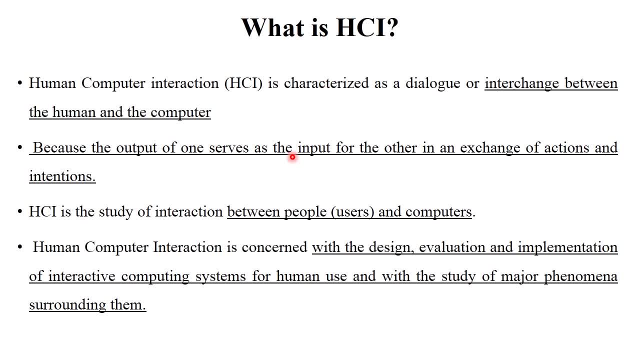 Now, first, what is mean by human computer interaction? right? So nowadays or in real life, each and every field, each and every organization, humans use the computers. right, There are different technical gadgets like computers, laptops, mobile, etc. So each and every interacted with that. technological gadgets: Okay, We provide some information to the computer. means we give input to the computer. 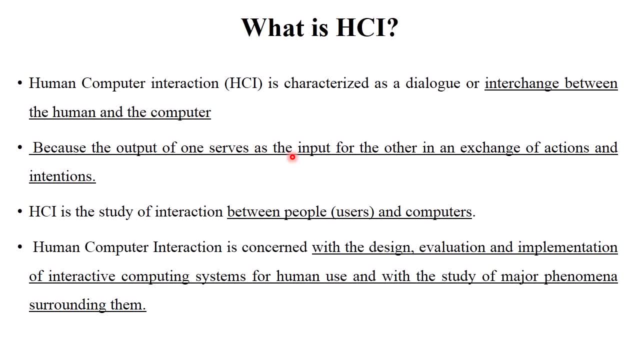 Right And computer provide us output. Similarly, vice versa, Computer provide us input and we provide us output Right. So this is called interchange, Clear. So this concept or this thing we used in our daily life. So human computer interaction simply means interchange between human and computer. Okay, And what is mean by interchange? means information interchange. It interchange the information between the computer and the human. Okay, 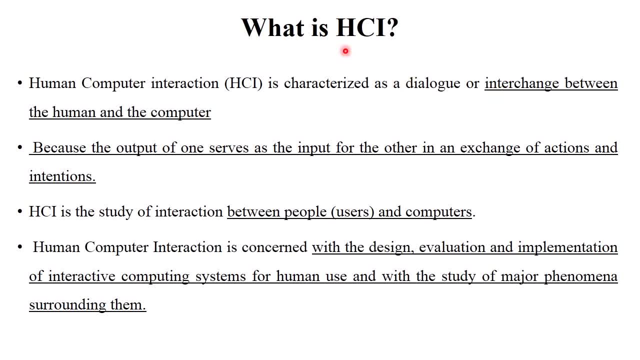 between human and computer, which is called as human-computer interaction right, Because the output of one serves as an input for the other in an exchange of actions and intentions. clear. So HCI is a study of interaction between people's, or we can say users and computers. 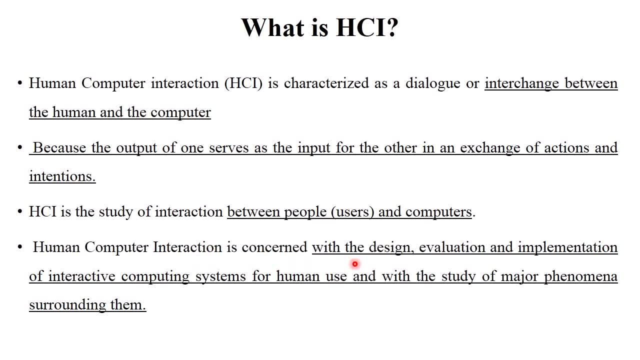 clear. So human-computer interaction is concerned with design, evaluation, implementation of interactive computing system of human use and with the study of major phenomena of surrounding them. okay, So this all thing which is called as human-computer interaction, So simply means: 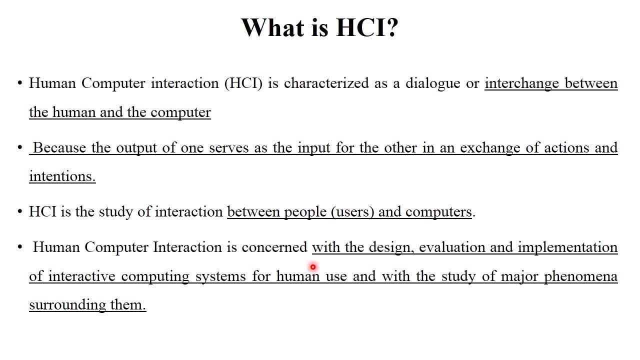 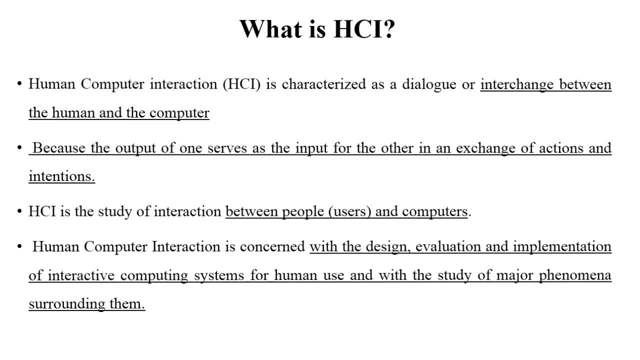 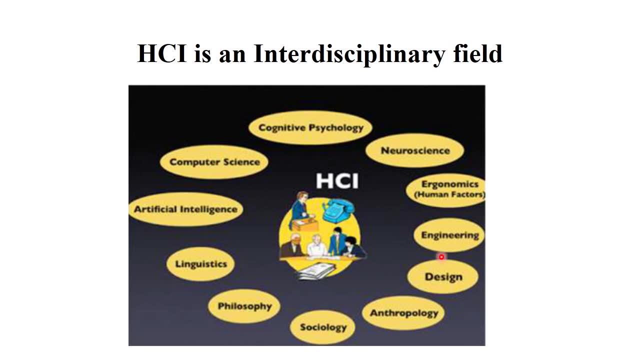 HCI means interchange information between human and computer. clear, So this is a concept of human-computer interaction. okay, Next now, human-computer interaction is an interdisciplinary field. See, there are fields of interaction between human and computer, right? So human-computer. 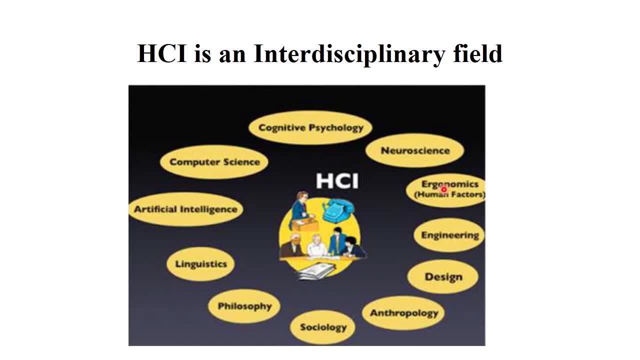 interaction is different field of interaction. So these fields are given, ie cognitive, psychology, neuroscience, ergonomics, engineering, design, then anthropology, sociology, philosophy, linguistic department, then artificial intelligence, computer science department. right, each and every field, each and every organization, computers are used or human is interacted. 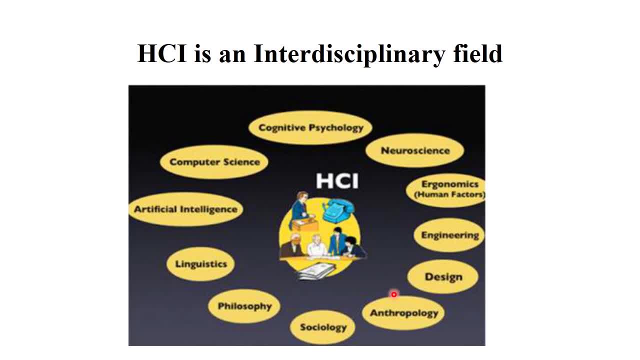 with the computers right. So these are the some fields where HCI is used. In my next video, we will learn in detail how HCI است führen ist And also- I hope you understand this- What is HCI exactly? in this field, essay is used. okay, this is just introduction of interdisciplinary field. 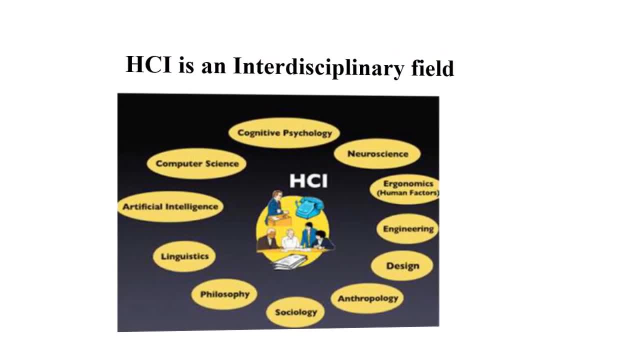 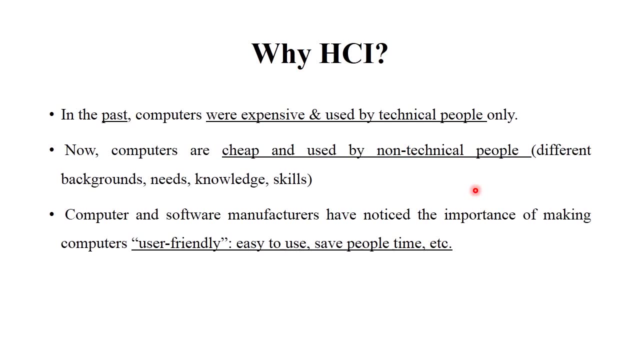 clear. okay, next now why human computer interaction is used. okay, we all know that human and computers- right, the gadgets, the technological things- are essential part of our life. okay, in the past computers were expensive, and which is used by technical people only. but nowadays computers are very cheap, which is used by non-technical people also. okay, the people. 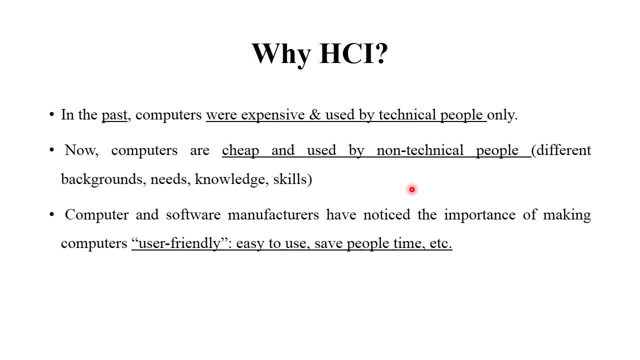 which has different backgrounds, different needs, knowledge, skills, the each and every people used computers, laptops and mobiles, etc. okay so computer is a need of technical and non-technical people also. okay so computers and software manufacturers have noticed all those things. so nowadays technical and non-technical people are very cheap, but nowadays computers are very cheap. 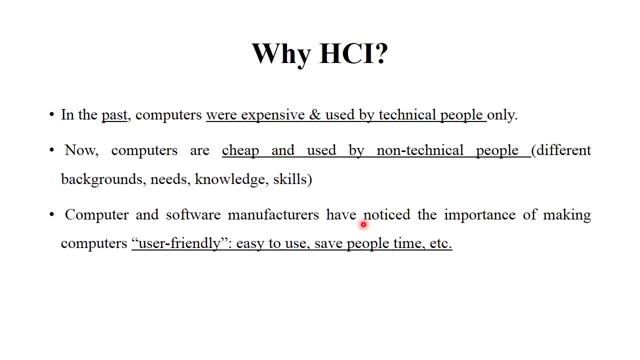 so these computers and software manufacturers make the computers more user friendly. okay, so what is mean by user friendly? user friendly means it very easy to use. it's more usable, flexible, okay, we can carry out laptop for each and everywhere which is portable, right it? and also we perform different operations by using mobiles, by using computers and laptops. so it? 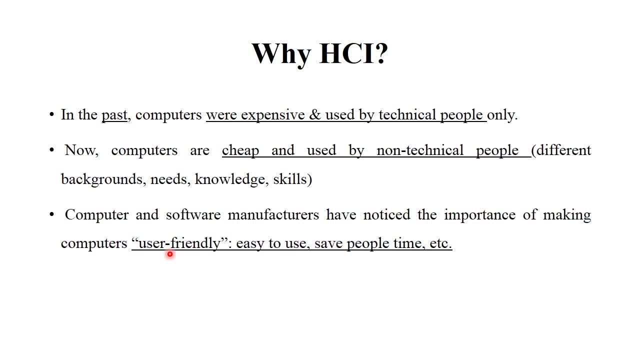 requires the people time. clear, which is called as user friendliness. okay, so that's why human computer interaction is necessary. okay, which provides solutions and also which helps the each and every organisation for their growth purpose. right, so that's why we use human computer interaction in each and every organization. clear, okay. there are some questionnaires about. 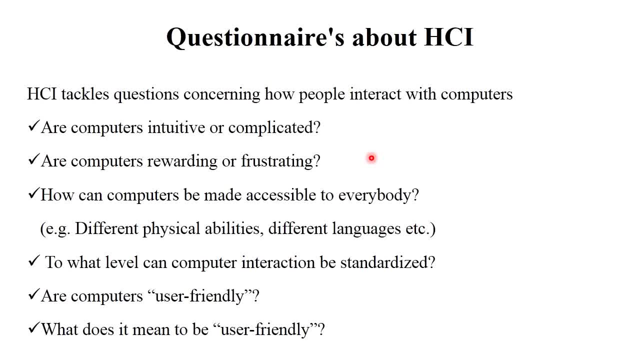 hcl. hcl is used for the research of Maurice Chir cách diyen apk. So here there is lots of coverage testing available. there is actually a lot of technical information cannot be documented from local government in the first place, which is really useful because about the reason. 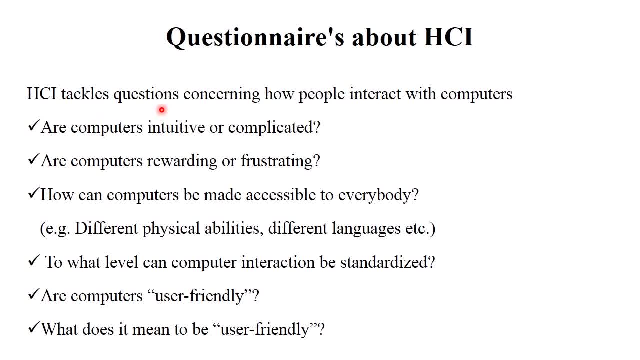 why webcomputing is interesting. it can cause about an amplitude ofSorry very specific. why webcomputing- Human computer interaction- tackles questions concerning how people interact with computers. Ok, So first question is: Are computers are complicated? What do you say about computers? are complicated? No, 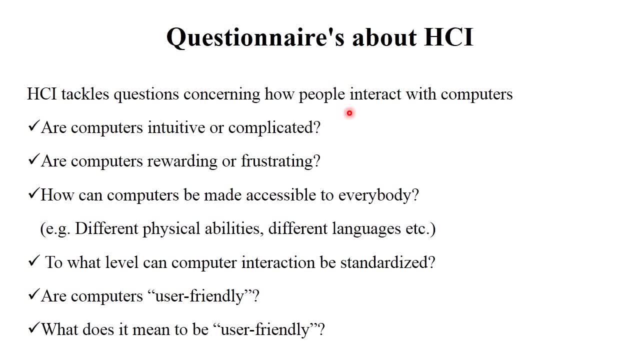 We all are familiar with that. The user friendliness is important. Clear. The next one is: Are computers is rewarding or frustrating? I think so. no, Computers provide solution for each and every questions. Clear Next: How can computers be made accessible to everybody? There are different physical abilities. 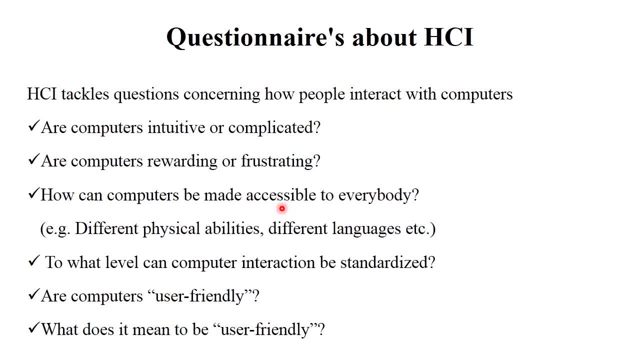 Different languages, Different religions And different countries Or different purpose. We used computers and laptops, Right. So how can computers be made accessible to everybody? Ok, The next question is: To what level can computer interaction be standardized? What is the standard of interaction? What is the standard of computers? 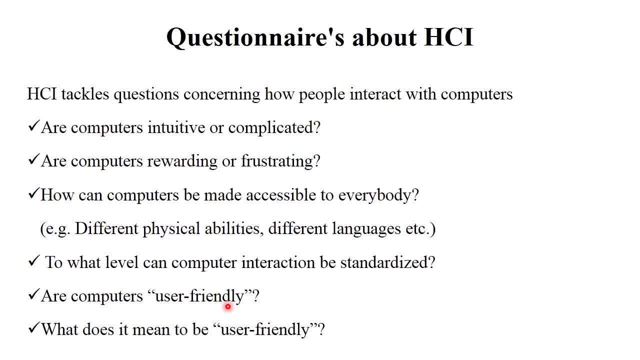 Right. The next question is: Are computers user friendly? What do you think Computers are user friendly? Yes, Computers are user friendly. We all are familiar with that, Right. And the last question is: What does it mean to be user friendly? User friendly means what? 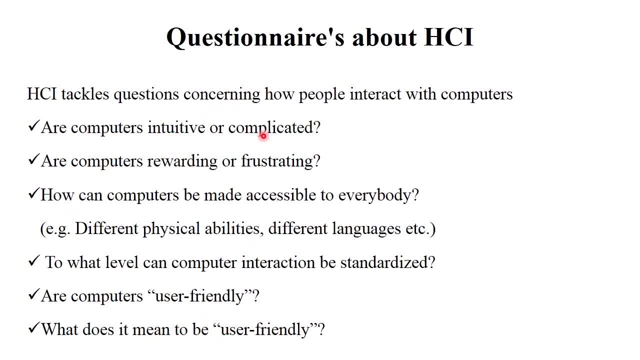 Ok, So these all answers of that particular questions are solved by human computer interaction. Ok, So this subject Human computer interaction gives answers of all those questions. Ok, So this subject human computer interaction gives answers of all those questions. Ok, In my next video We will learn about in detail. 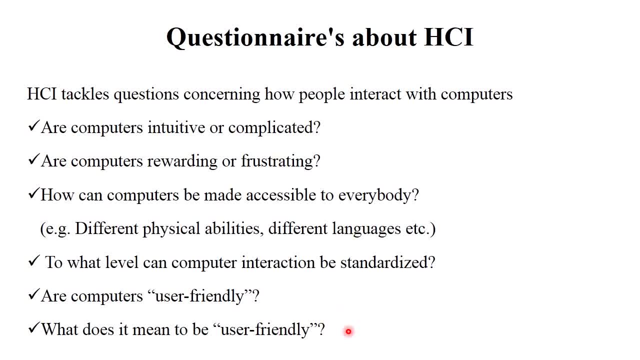 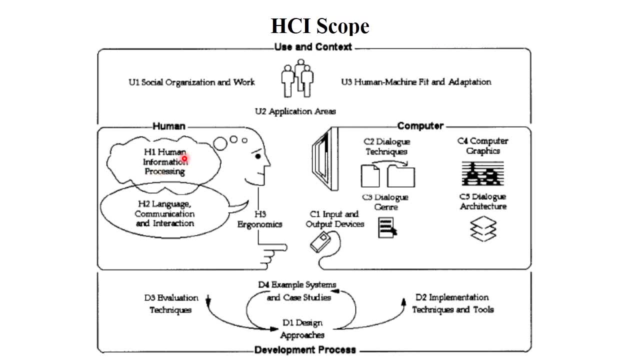 The answers of that particular questions Clear, Ok. Next Now HCI scope. So see, here This is human And this is computer. Ok, Let's consider that Human have some social organization and work, Ok. And the computers means Human, machine, fit and adaption. Clear. So Human used The computer. 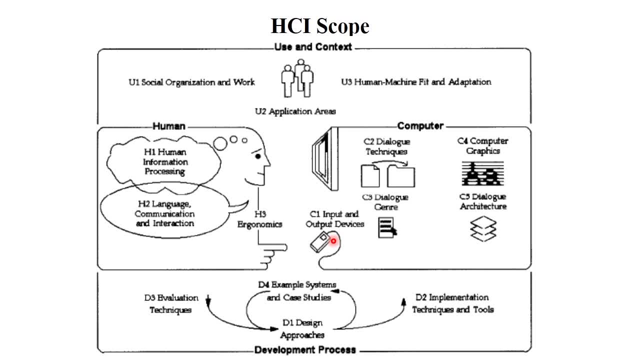 Right By using some input devices and output devices. Clear Human use mouse keyboard for handling the particular computer. Right Human provide some input to the computer And computer provide the output to the human. Clear. So human has some human information processing in their brain. Right- Human has different language, communication and interaction. 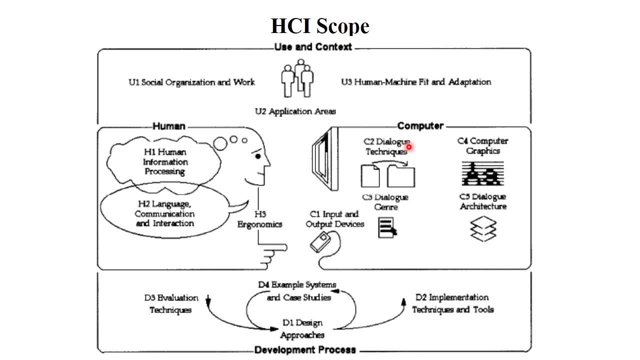 Clear. So human provide some input to the computer and computer provide the output to the human. 5. Computer has different dialog techniques. Right, So how computer can give input to the computer. It has different dialogue techniques: A- Dialogue generations, A- Dialogue architectures, B- Dialogue graphics. 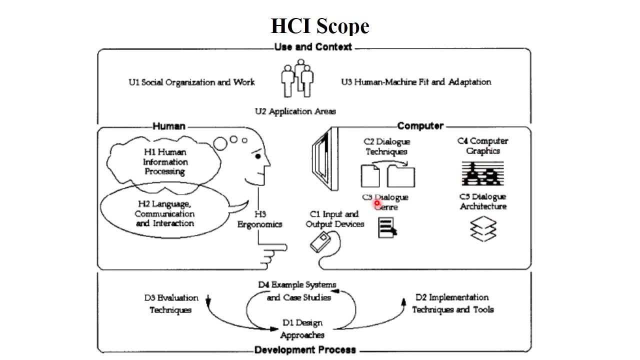 C. Ap 책 C- Operating system, D Specifications, C Interfaces D- Back interface, D Sheet E- Front and back interface, C Interfaces. So when human give particular input to the computer, Computer gives the output on that particular screen. Ok, This is called user interface. 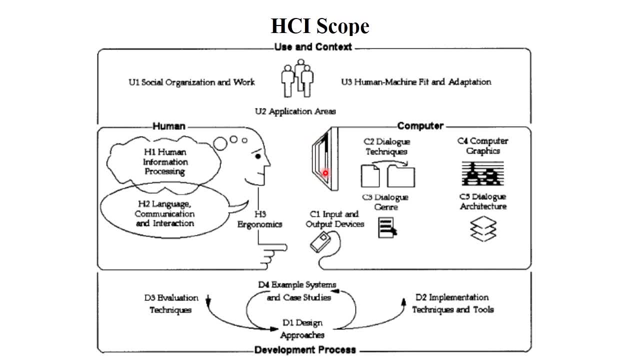 Computer has two interface: Front interface and Back interface. Ok, How exactly computer work. Ok, this is backend or back interface, right? and what exactly the output? this is the front interface: clear, so human is interacted, more friendly to this interface. clear, so this is called human and computer interaction. clear, so human. 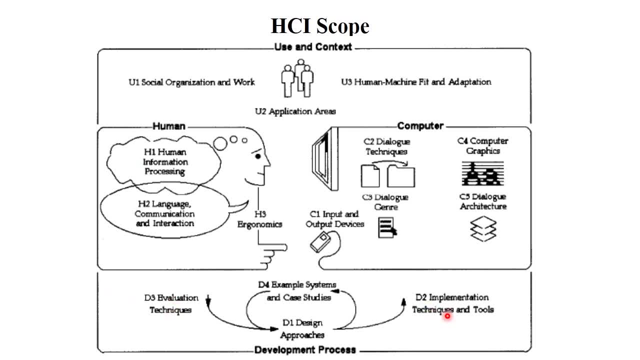 has different evaluation technique. computer has some implementation techniques and tool. okay, obviously computers are made by human after all, right, so computer use different evaluation techniques for implementing the products right and gives proper output in that particular screen. okay, so this is called development process. okay, and in this process multiple users are. 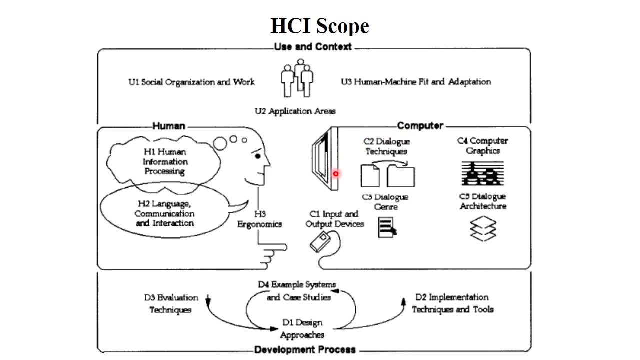 involved and multiple systems are involved. clear, so this is a scope of HCI, where human computer interaction is used. okay, so this diagram shows that the development process, user and context, what exactly human thing, what exactly computers are done. okay, so this, all things are shown in that particular diagram. so this is called HCS scope. clear. 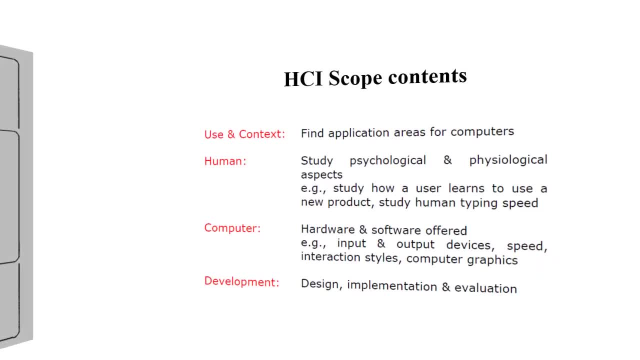 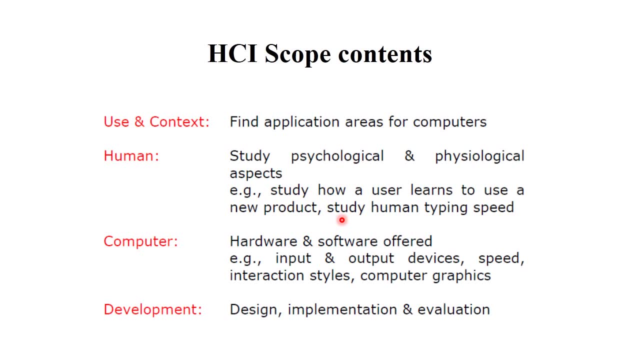 okay, HCS scope contents. in previous diagram we will learn the particular methods, how users are interacted with the computers. okay, so this involves four contents, as is user and context, human, computer and development. right Use and context means find application areas of computers What exactly perform or what operations are exactly perform by the computer. 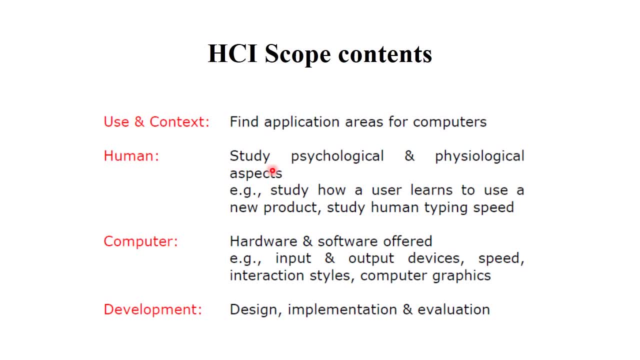 Clear. Next, human Humans: study all psychological and sociological things or aspects. Okay, For example, study how a user learn to use a new product And study human typing speed. Clear. This is a study of human Right. Next, computer: Computer means hardware and software offered. 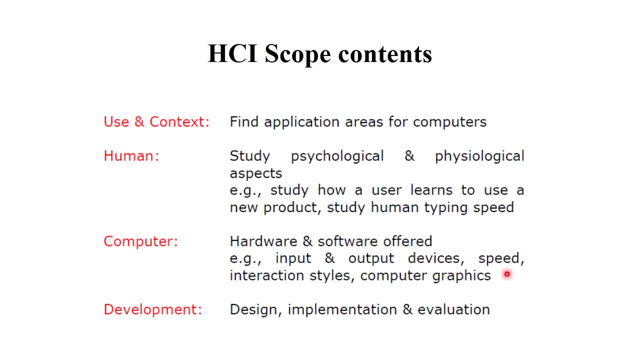 Okay, For example input and output device speed, interaction styles, computer graphics, etc. When you provide a particular input in instant way or in the second, Computer gives the feedback or proper output Right. So this is the interaction speed of that particular computer. 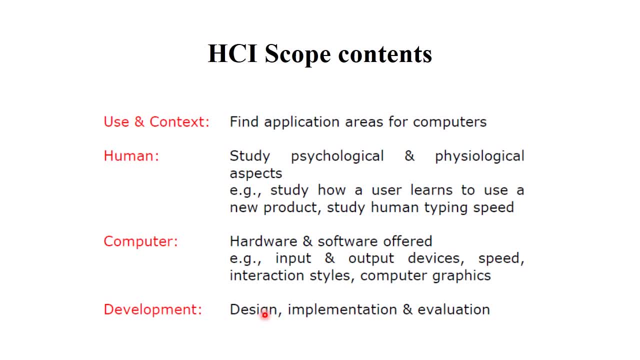 And last, development. Development involves design, implementation and evaluation- Clear. So how exactly Human processor is used, computers and development- We will learn in my next video. Okay, This is just introduction of HCI. scope contents- Clear. Okay. Next, This is the components of HCI. 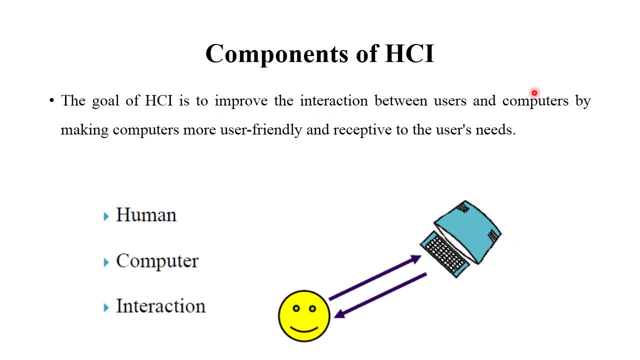 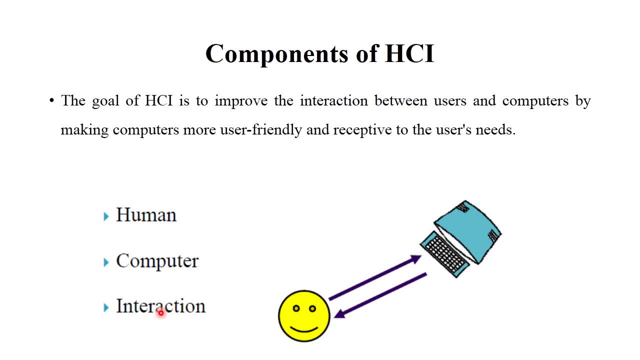 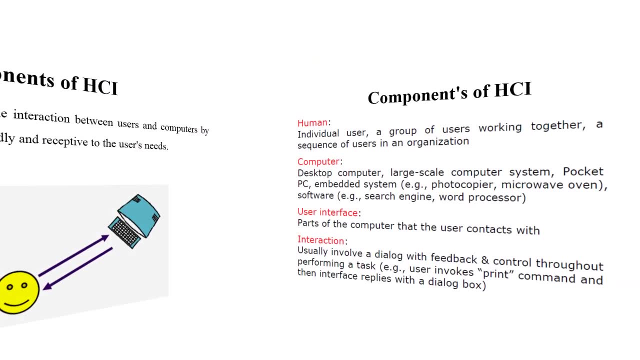 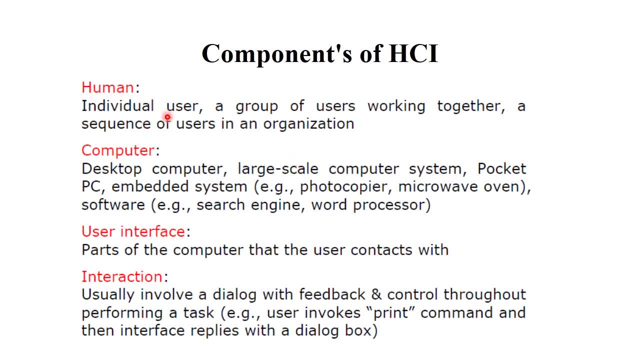 What exactly mean human? Human means individual users, group of users. they are working together, Okay. Or sequence of users in an organisation: Clear, Okay. What do you mean by computer? Computers means desktop computer, large-scale computer system, embedded system, computer-based systems and private system. 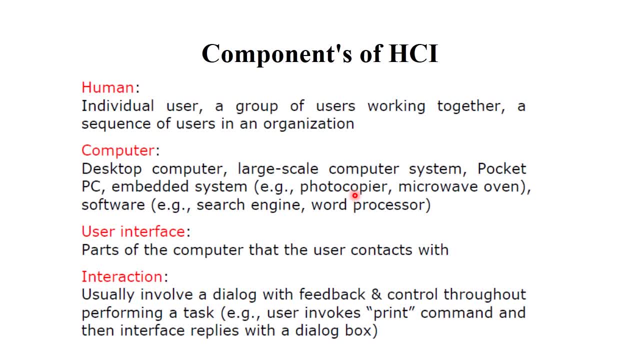 Also there are some technological things like photocopy, microwave, oven, etc. Also there are some softwares like searching engine, word processors, etc. Each and every application we will install in our computer or laptop or mobile, which is called as technological gadgets. 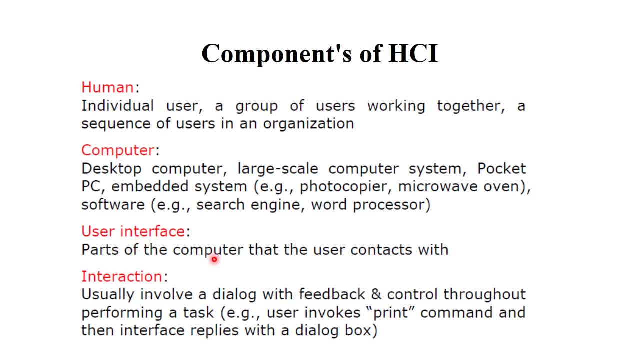 The next is user interface. User interface means part of the computer that user contact with. I already tell you front interface and back interface, So user interacted with the computer by their front interface. And last interaction Usually involve a dialogue with feedback and control throughout the performing task.